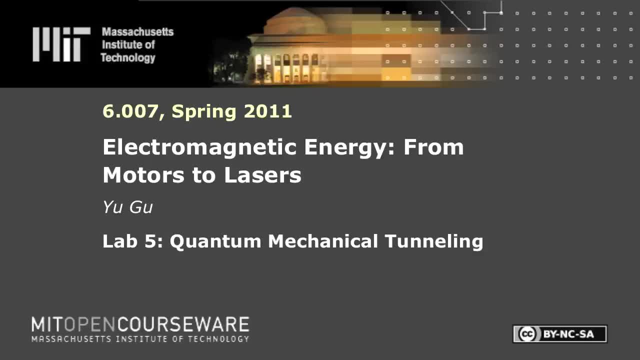 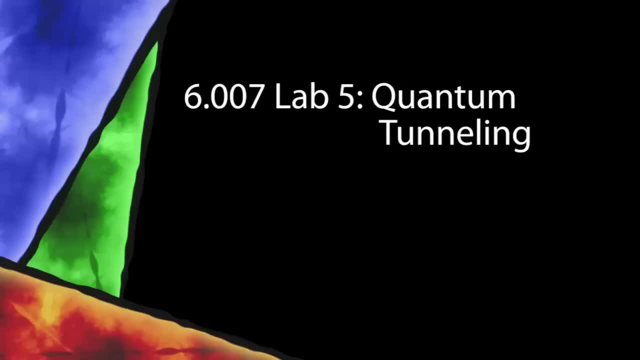 Welcome to Lab 5, Quantum Mechanical Tunneling. In this lab you will be characterizing a rubber-nickel compound called Quantum Tunneling Composite or QTC. You will be using it to make a touchpad. This lab requires the use of a 5 volt high current power supply. Let's 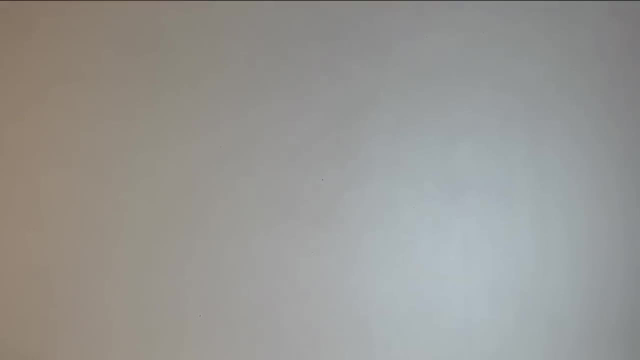 go over the additional components For this lab. you will need copper tape, double-sided tape, three glass slides and one glass slide coated with ITO. about five pieces of the QTC material, some ball bearings, rubber strips which act as spacers. 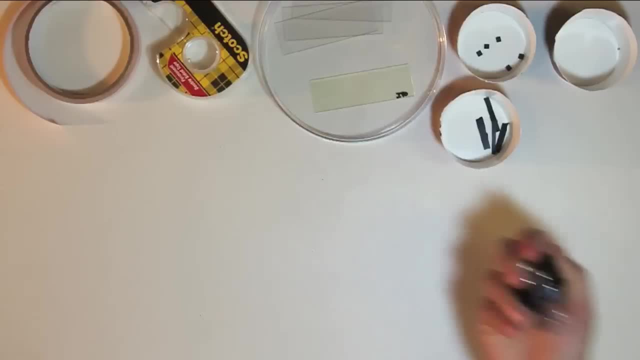 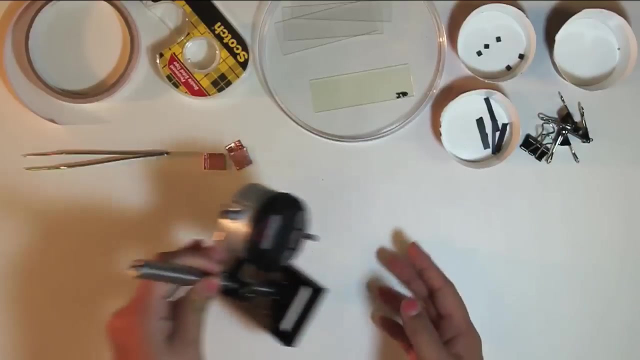 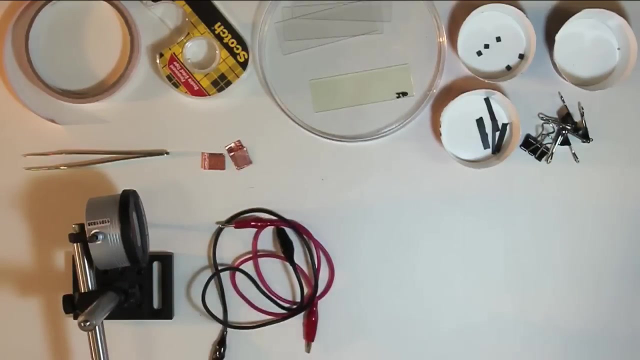 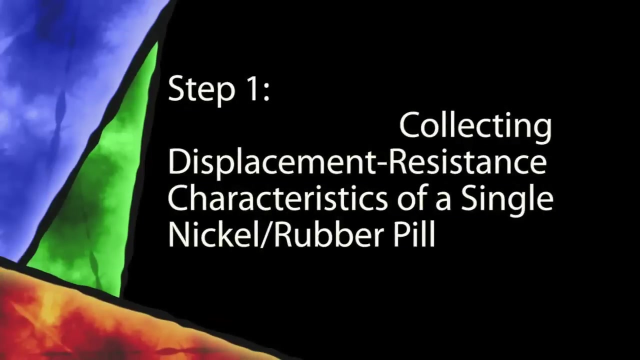 Binder clips, some tweezers, two pieces of glass coated with copper- these act as electrodes- a sensitive displacement gauge. finally, some alligator clips and a multimeter For Part 1 of the lab. you will be measuring the displacement versus resistance curve of 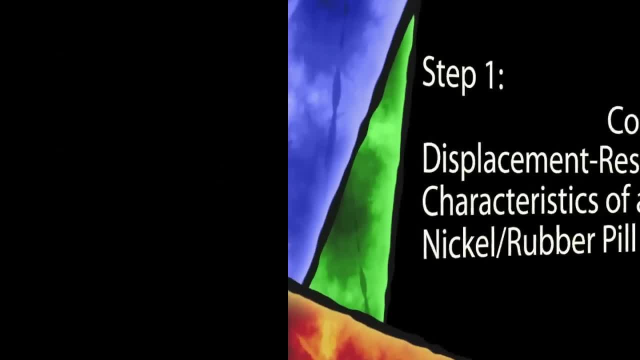 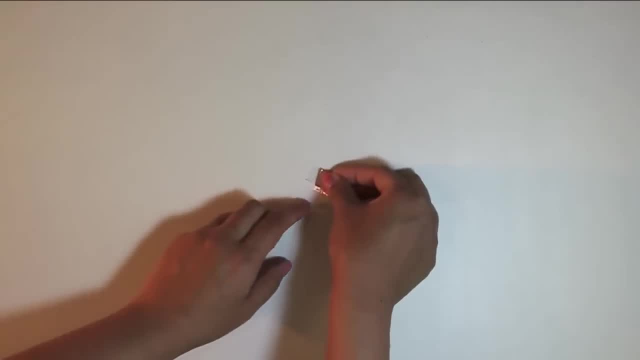 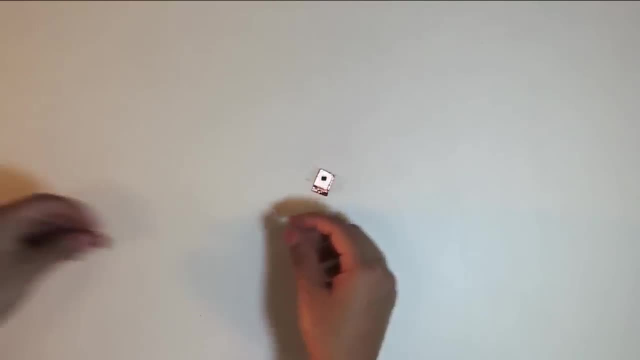 the QTC pill. Begin by placing a copper electrode on the table and attaching it with double-sided tape. Place the QTC pill between the two plates. Place the QTC pill between the two plates. Place the QTC pill between the two plates. 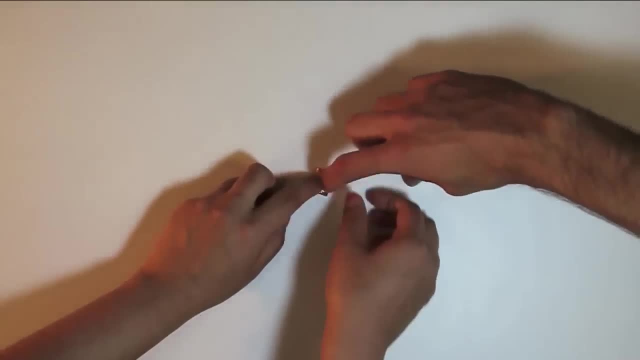 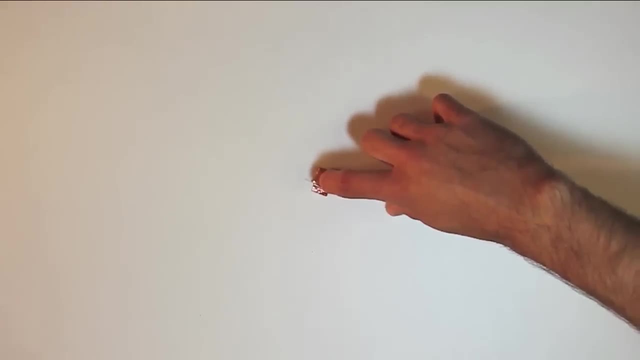 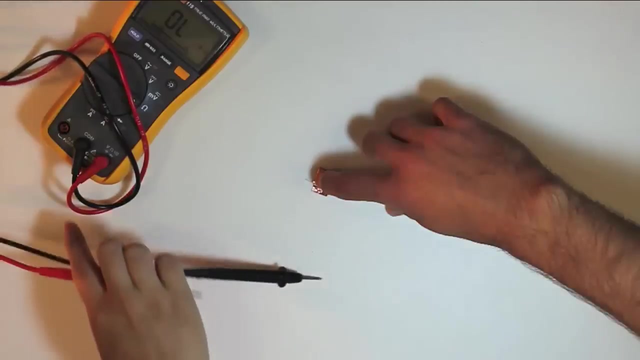 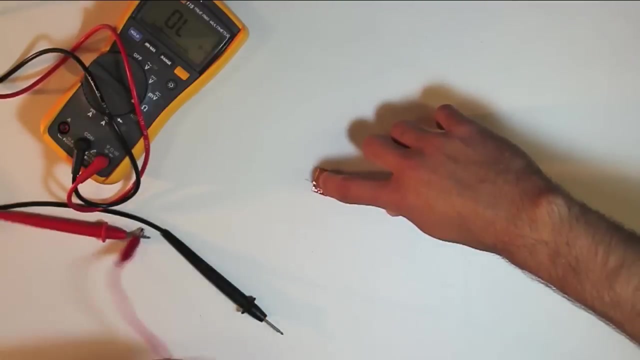 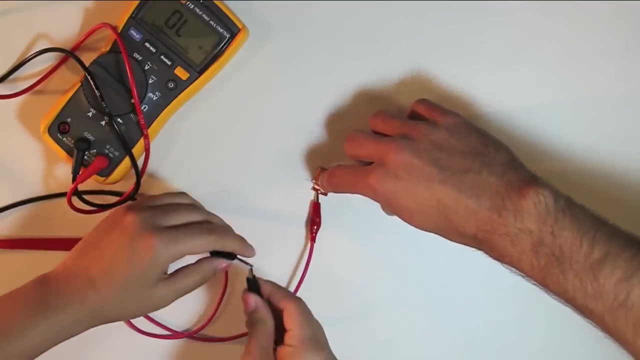 Place the QTC pill between the two copper electrodes and hold it in place. Set your multimeter to measure resistance and connect it to the top and bottom electrodes. You can also touch the QTC-Sammler together, but you'll have to place theouring on both. 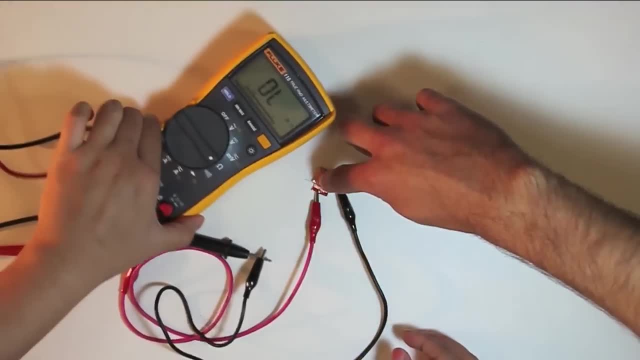 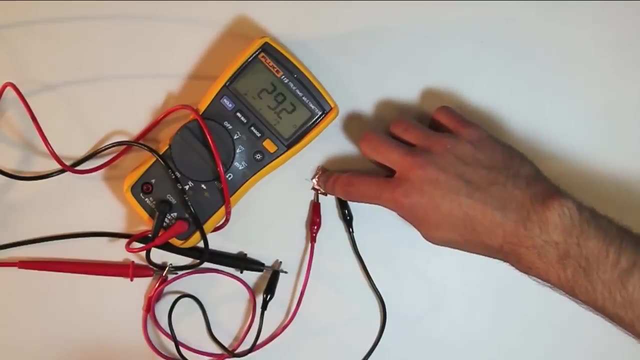 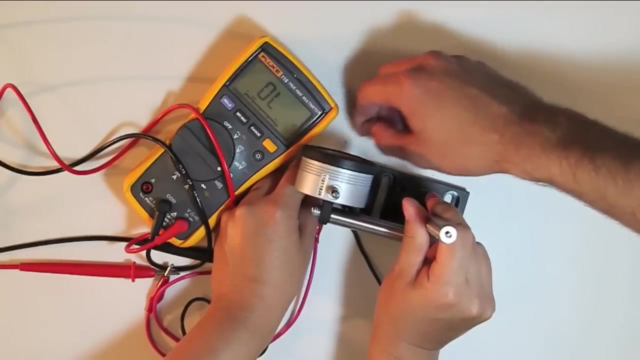 points and also shake it with the communauter Press to adjust the QTC-Sammler. Now tune theopl 핑. You are ready to set the reclaiming retardant. Like this, you can Cool the Now position this device on top of the QTC pill, which is sandwiched between. the electrodes. You can now measure the resistance with the instruments. ich 먹 안에 quartzo punto. you can now measure the resistance and the calcium Pooleman redemption in theluisa array to determine which electrode is in lack. of sugar by zwicka is in baby blue. 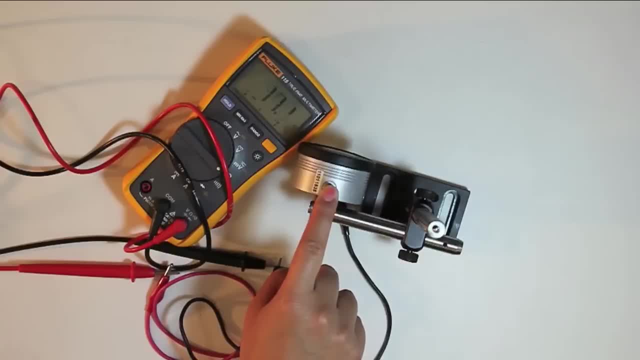 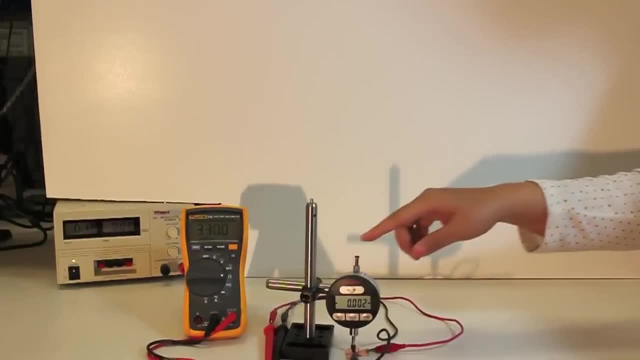 panels with Fentanyl are important of the QTC pill as you press down on the displacement gauge. Here's the same setup from the side view. As displacement or compression increases, resistance should decrease non-linearly. This should make a straight line on the log-log scale. 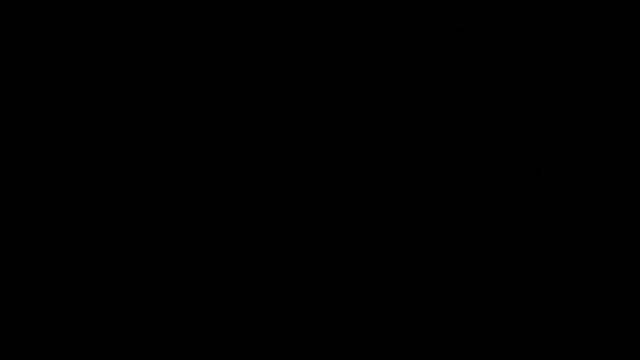 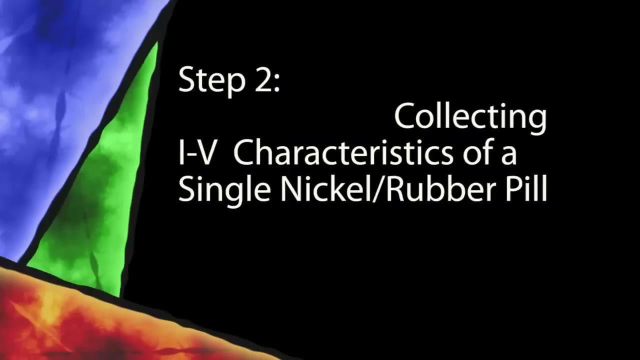 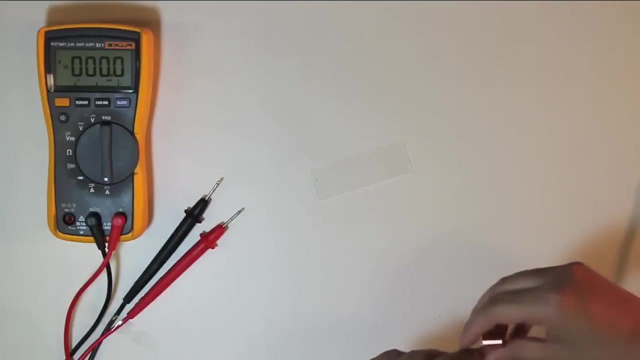 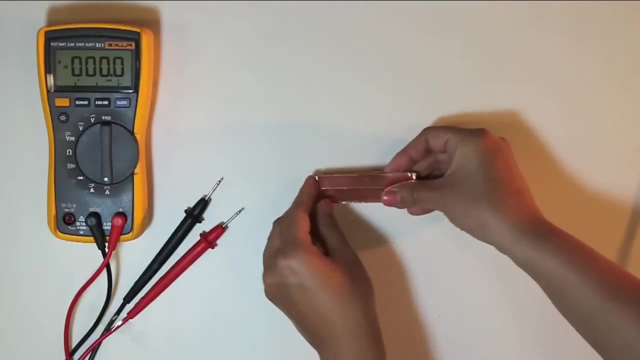 Part 2 of the lab will be measuring the IV characteristics of a QTC pill. We will use two glass slides to make a more advanced pair of electrodes. Begin by covering one glass slide entirely with copper tape. Attach a third piece of copper tape as shown in the lab handout. 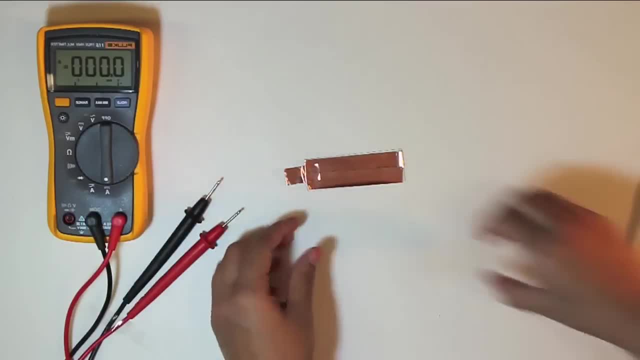 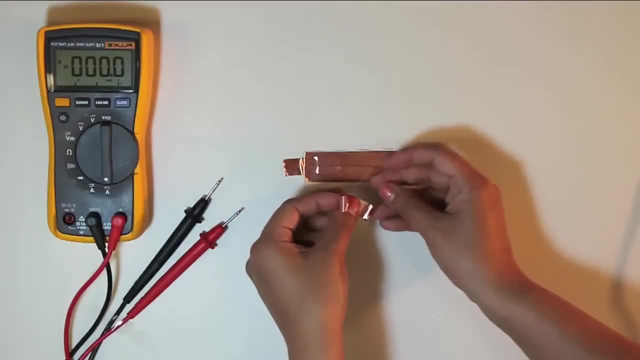 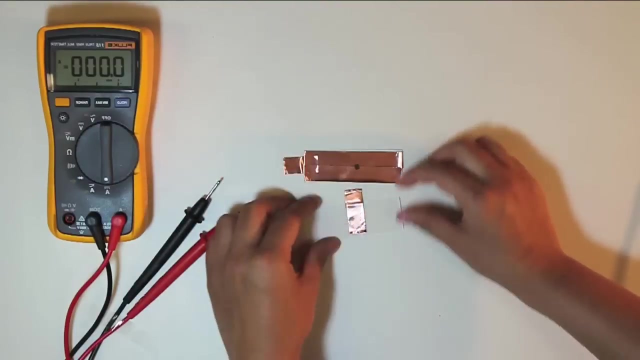 With the second piece of glass. attach a single piece of copper tape to the second glass slide. Place the QTC strip orthogonally. Place the QTC pill near the center of the glass slide so it makes good contact with both pieces of copper. 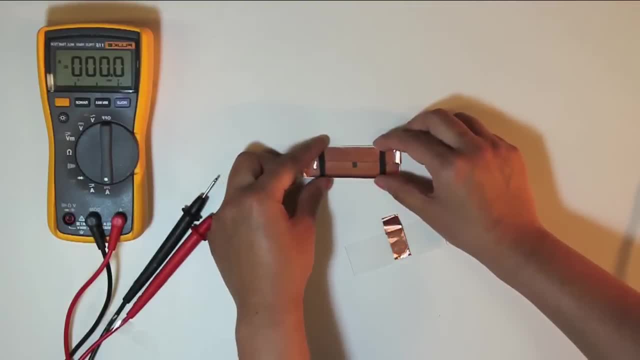 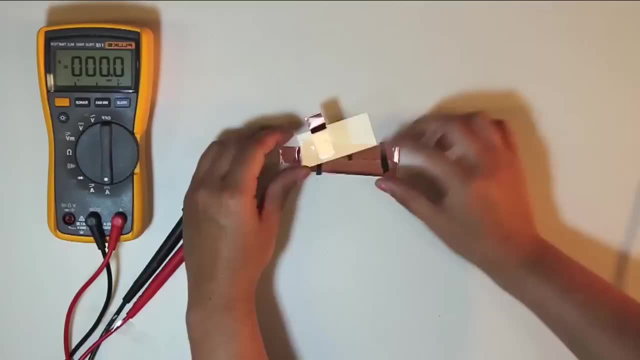 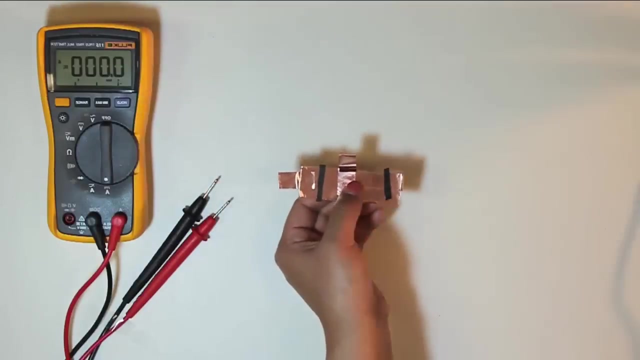 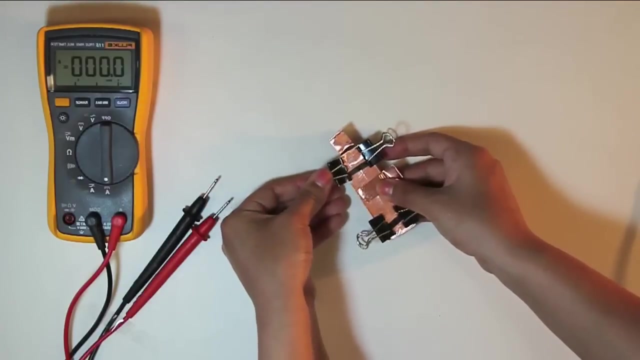 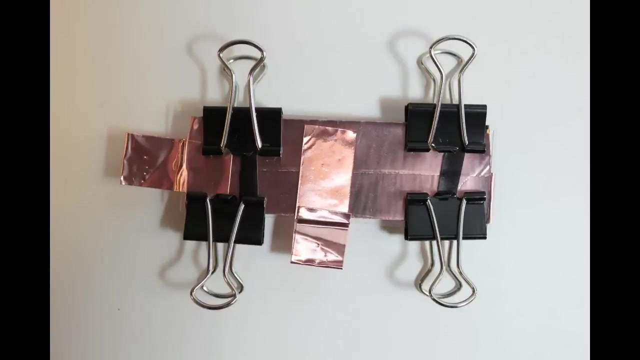 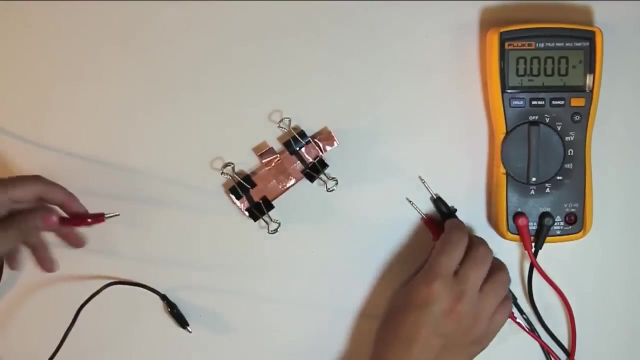 Add rubber strips for spacers. Finally, finish your setup by adding binder clips. Finally, finish your setup by adding binder clips. Add rubber strips for spacers. Here's a close-up of the finished assembly. Connect the power supply. Connect the multimeter in series so that it can be used to measure current as you apply. 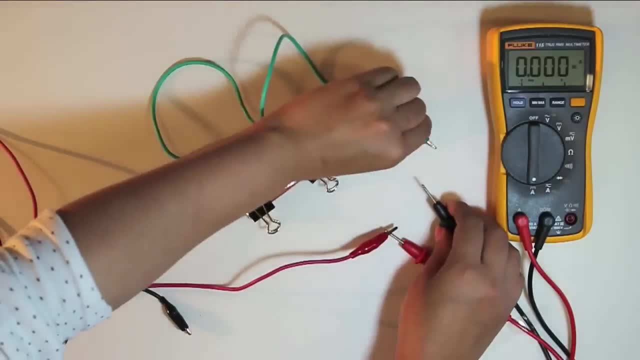 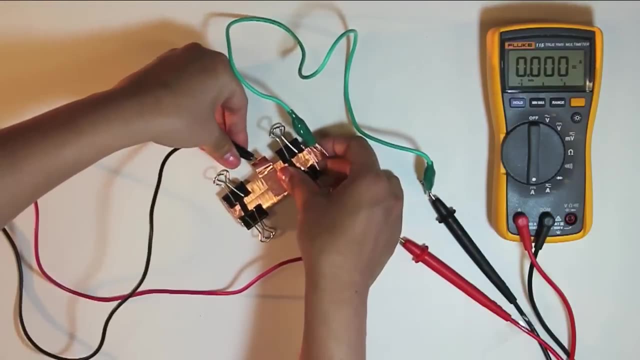 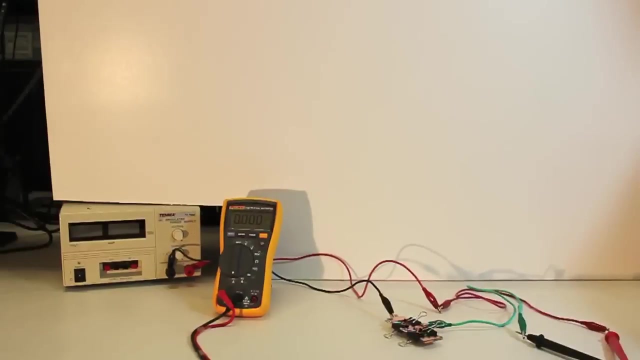 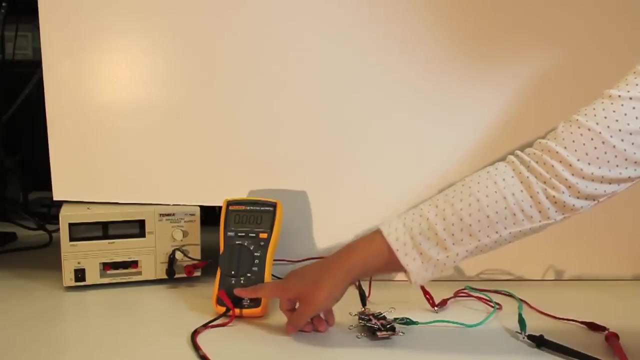 different voltages across the QTC pill. Here's the same setup from the side. The power supply is connected to the input of the multimeter, right now acting as an ammeter. The output from the multimeter is connected to the input of the QTC assembly. 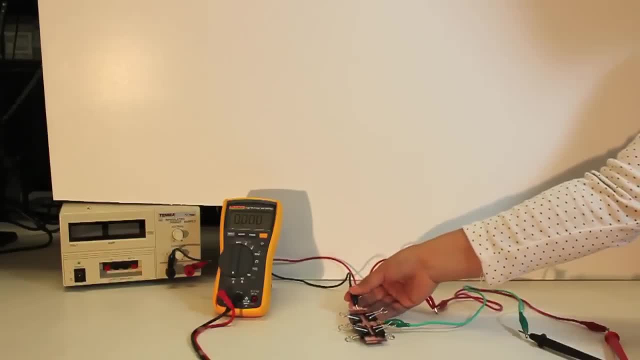 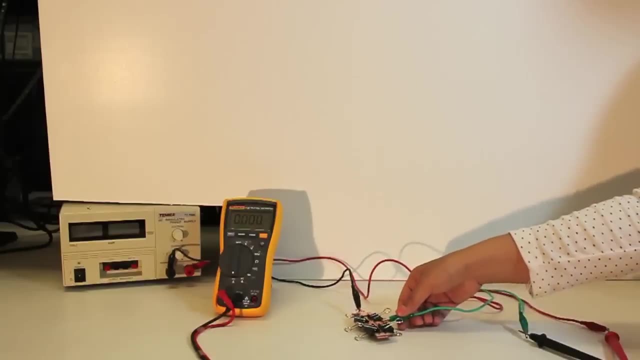 Okay, Finally, the QTC assembly is grounded to the ground of the power supply. Because we do not want to keep current across the QTC for long periods of time, we will begin by opening the circuit To make an I-V measurement. first, set the power supply to the desired voltage. 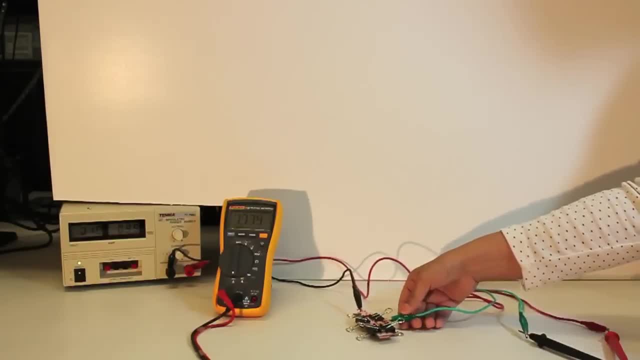 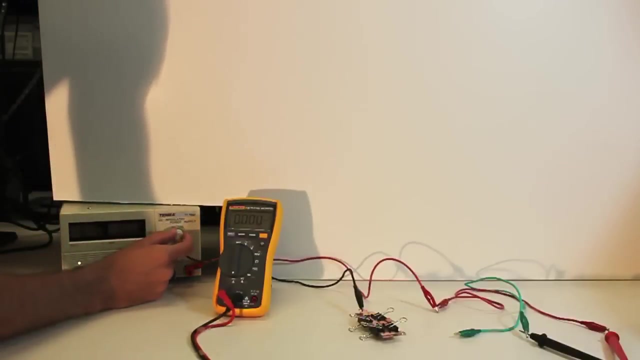 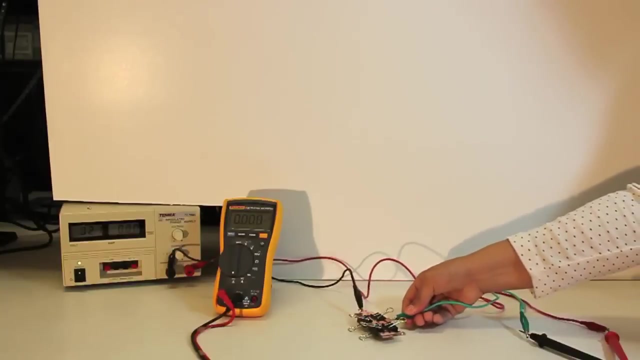 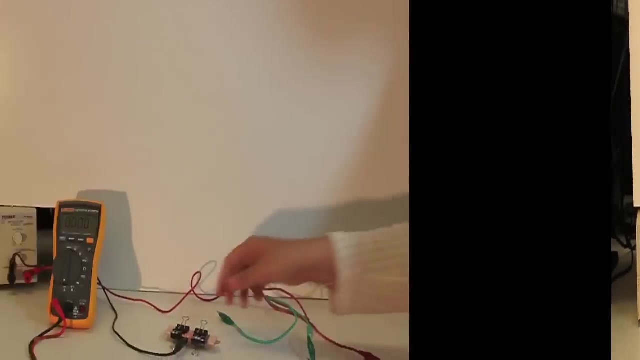 Connect the circuit briefly and take the reading from the multimeter. Repeat this for each voltage documented in your lab handout. Then release the power supply to the ground of the QTC раз. Take out the power supply close to you and connect it to the QTC preemmetry. 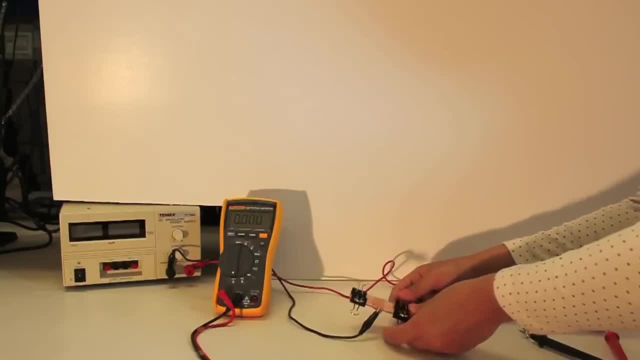 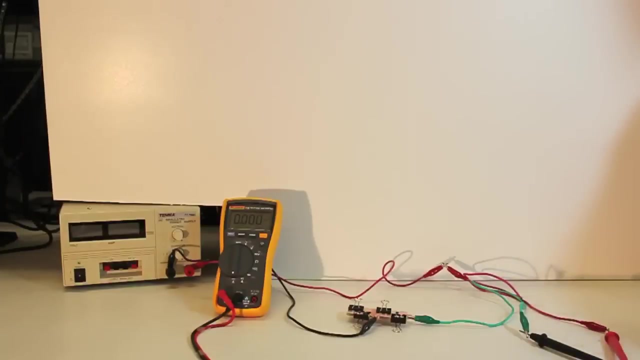 Push the power supply before the special switch. Eddie always works, unlike everyone else. Hold the plug for five sharpnels, fix it with a key and re-take as much voltage as you can with the adapter signed this down and make sure the disputed voltage is completed before relating it to. the conductor's普E clue board Open survival in q-tel and then call D茶 en plano in parallel Timing. now, 이 Mate, There are two options in my disparities in conseguences. There are two options for primary asteroid occupancy: one dedicated by Paul Gabbard and 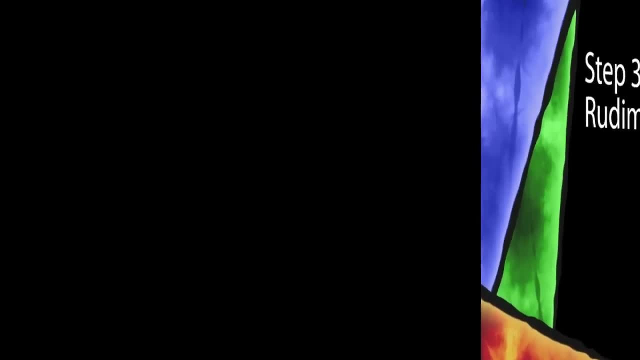 using a brightest alpha and different parameters available for Saintителя and laser. outer Kos, JENULS. Bye everyone, Good luck, Bye everyone, Bye everyone. The bottom half of the assembly has an electrode that's identical to what is made in Part 2.. 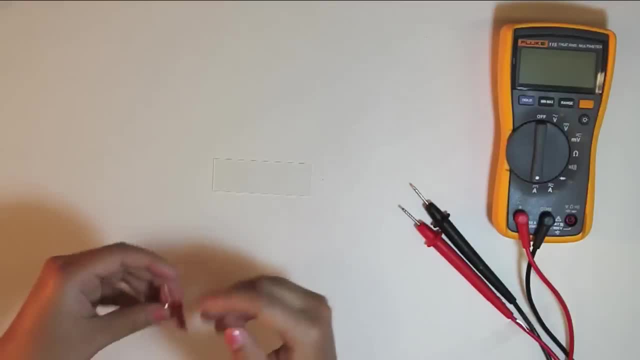 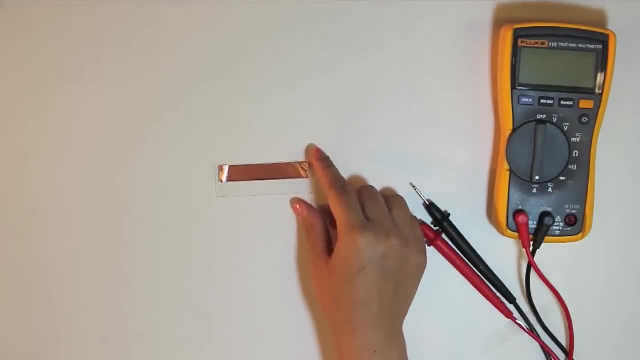 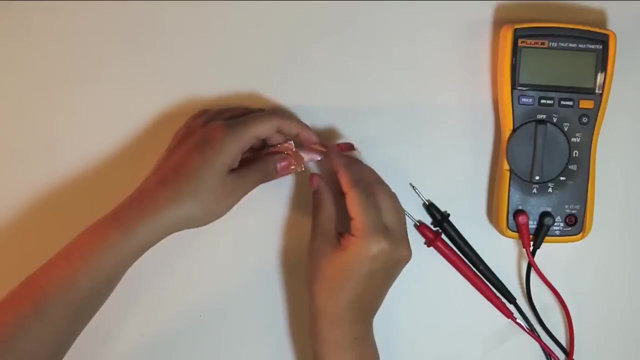 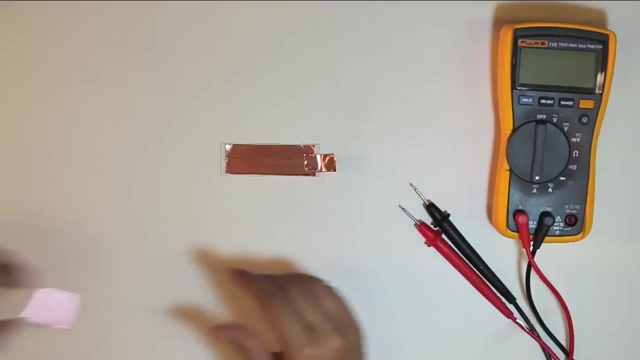 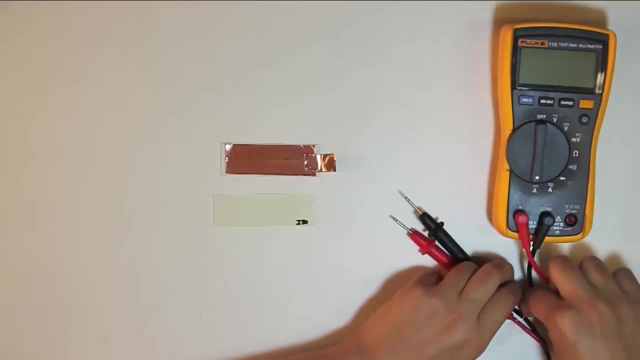 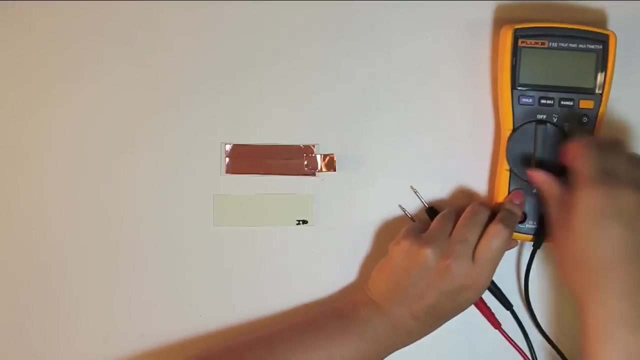 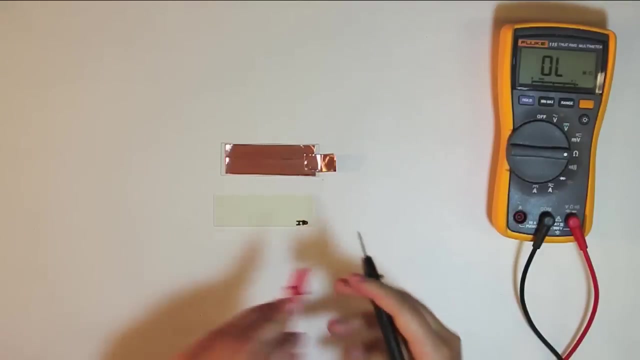 Place copper tape on one of the glass slides. Add a third piece of tape to make it easy to attach the alligator clips. The top half of the assembly will be made using a piece of ITO coated glass. The side of the glass with ITO should be marked, but if you're unsure, you can always test this with the ohmmeter. 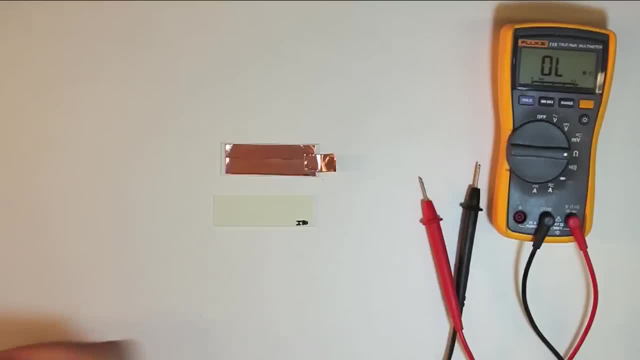 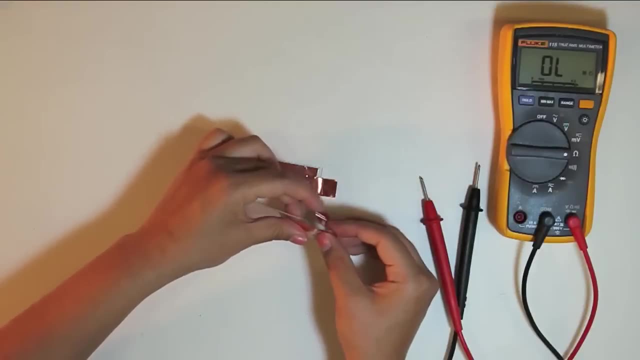 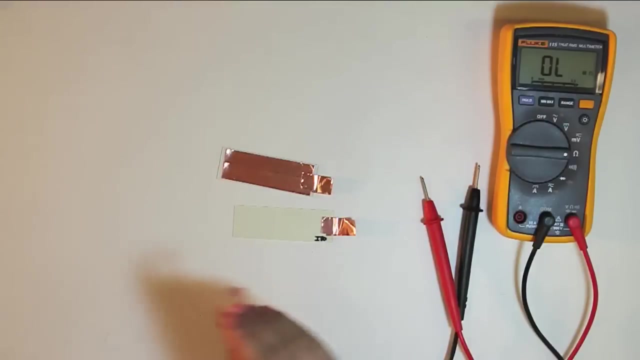 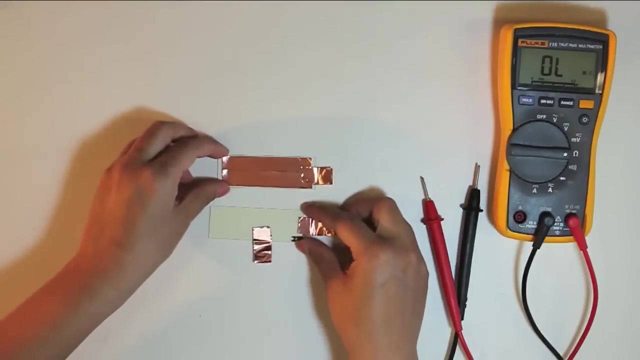 Place two pieces of copper tape as detailed in the lab handout. The top half of the assembly will be made using a piece of ITO coated glass. Place the other piece of tape, as detailed in the lab handout. The top half of the assembly will be made using a piece of ITO coated glass. 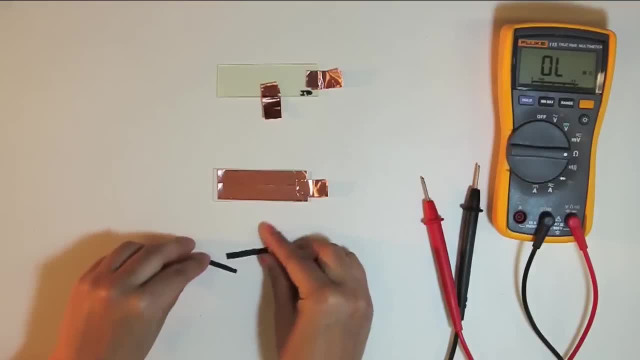 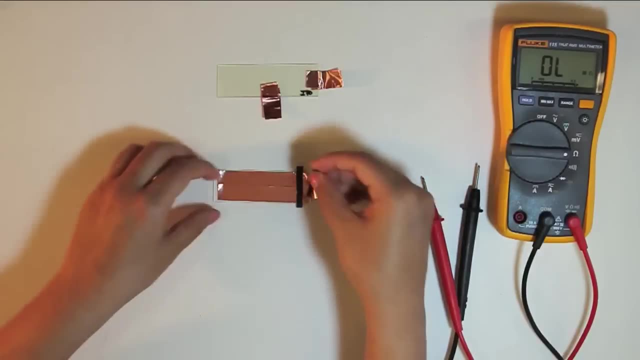 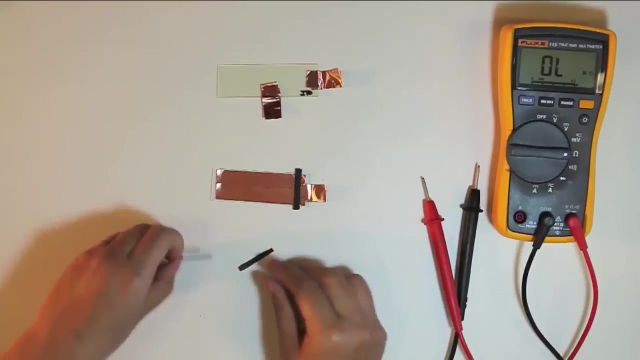 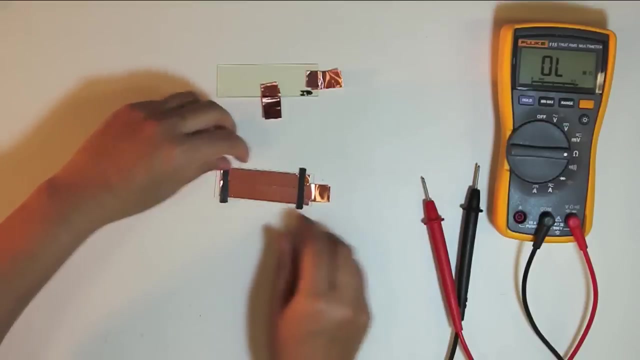 Now put four rubber strips to act as spacers. Then place four pieces of QTC pills in the four quadrants of the slide. Then place four pieces of QTC pills in the four quadrants of the slide. You will put ball bearings on these QTC pills. 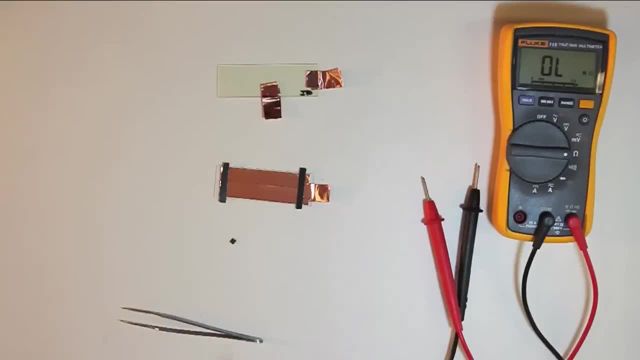 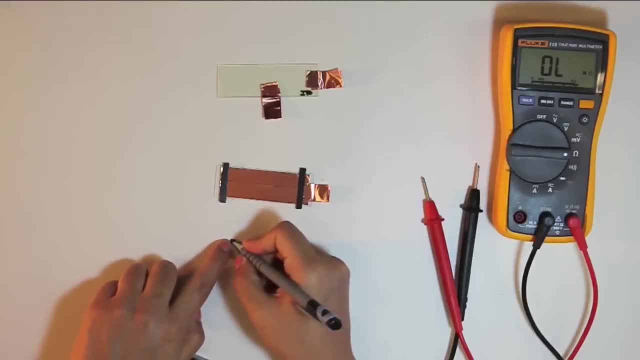 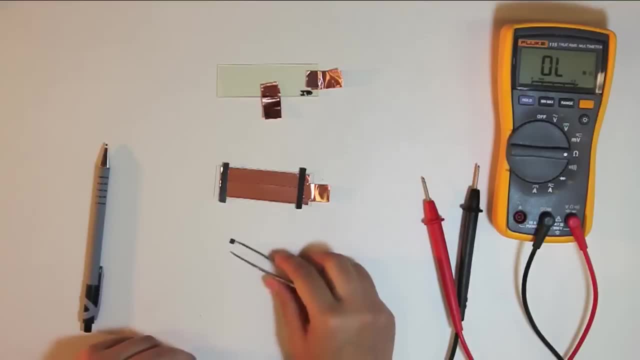 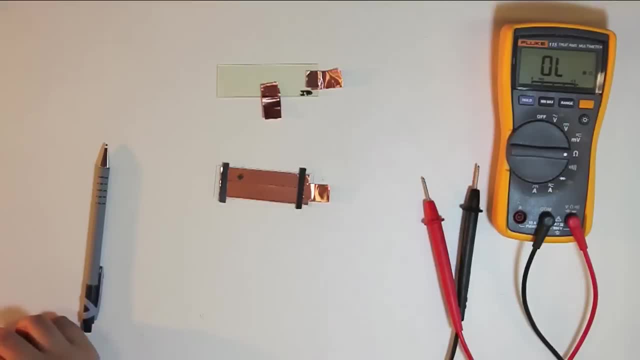 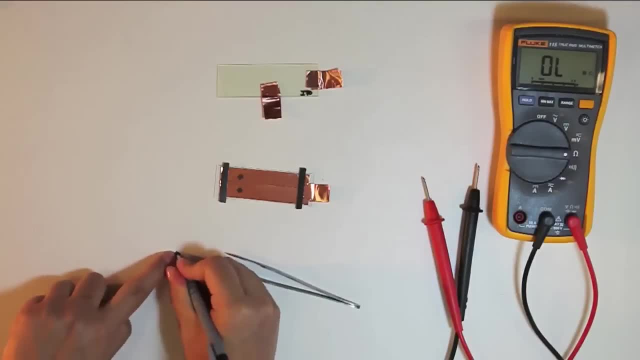 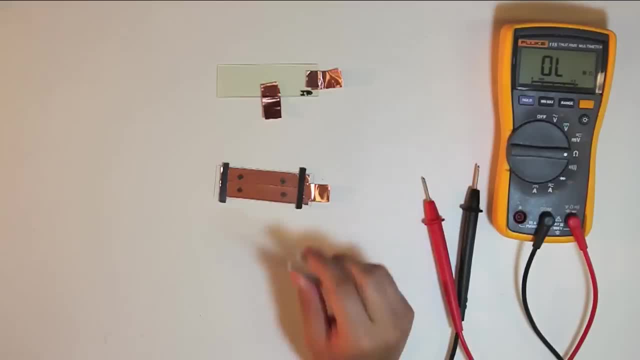 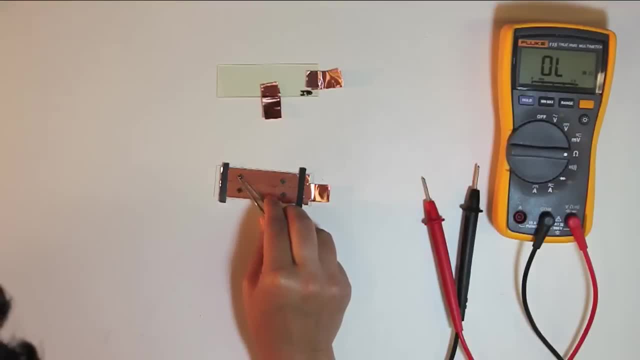 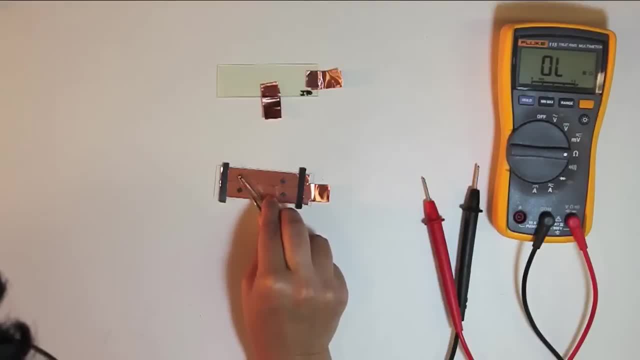 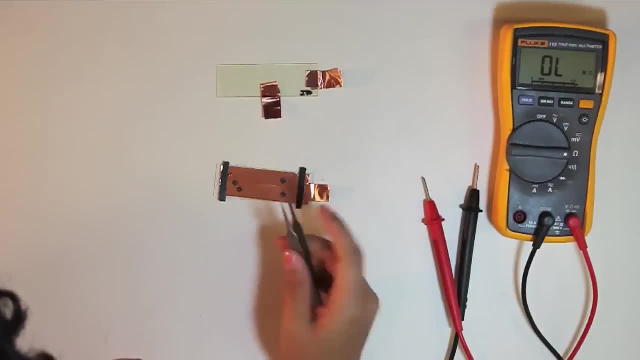 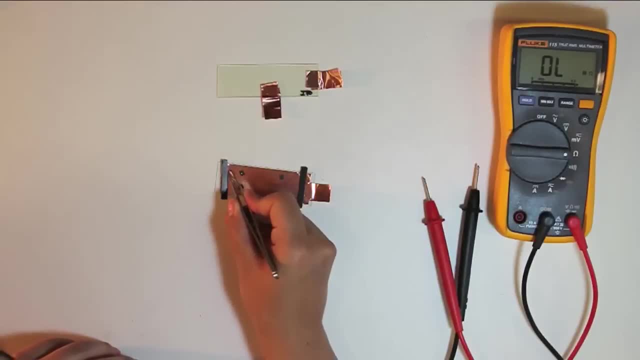